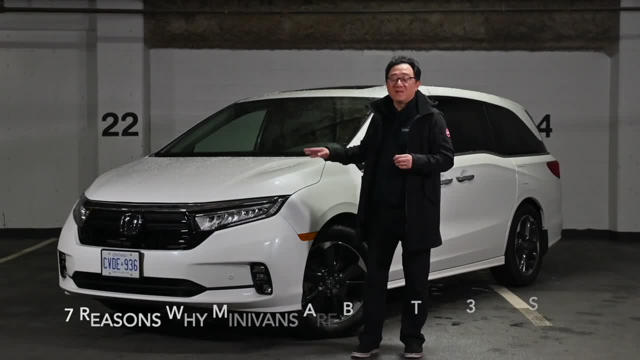 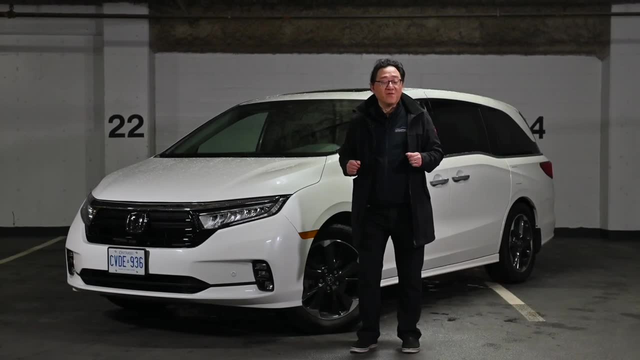 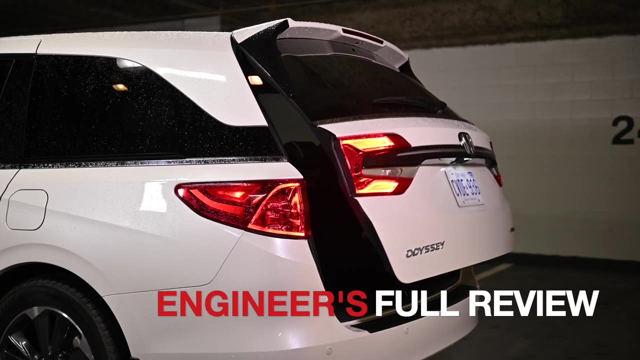 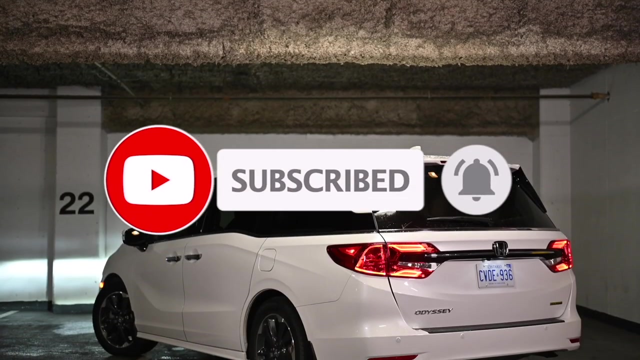 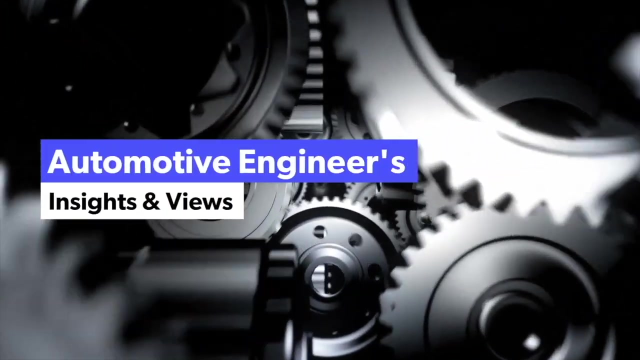 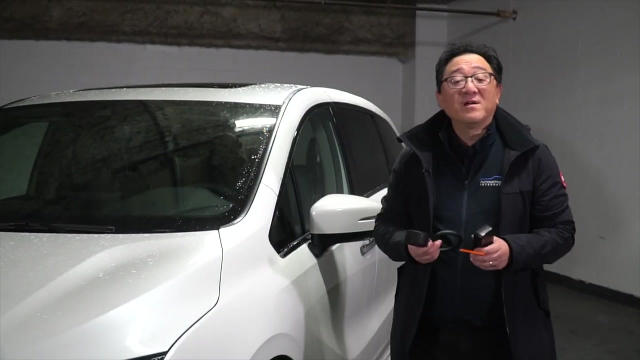 So let me give you seven reasons why I think minivans such as this Honda Odyssey is simply better and more practical and makes more sense than your traditional SUVs and crossovers. Okay, so I am going to talk about why I think minivans makes more sense than SUVs. 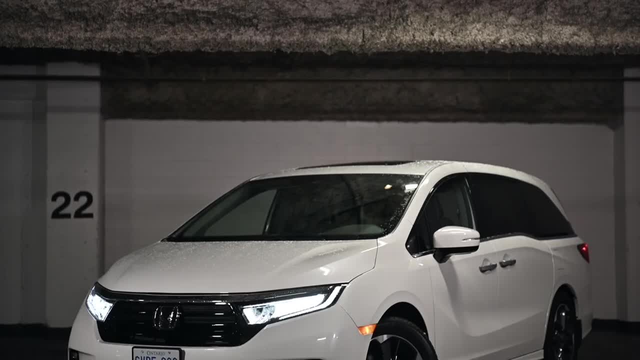 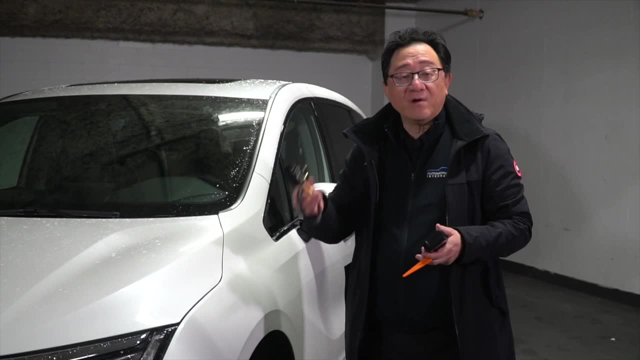 and crossovers. But before I do that, let's do a quick engineer's audit on this new 2022 Honda Odyssey, which I'm really enjoying. I'm going to first of all make sure that the tire pressures are okay. So I did that already and adjusted the tire pressure for all four tires by about two PSI. 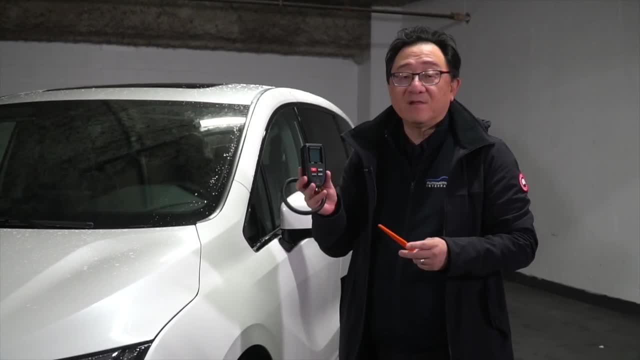 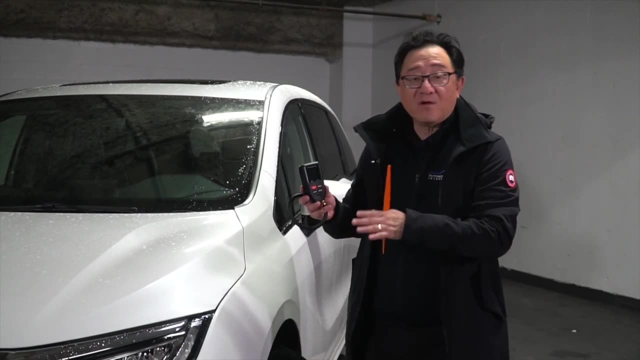 or so. So that's all adjusted And I'm going to do my usual paint check, which is using a paint thickness gauge to see if the quality of the paint is good and whether there's enough paint on the car. And finally, I'm going to do a quick body check to see what the 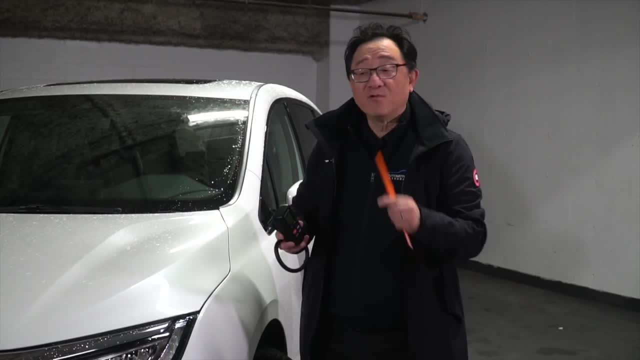 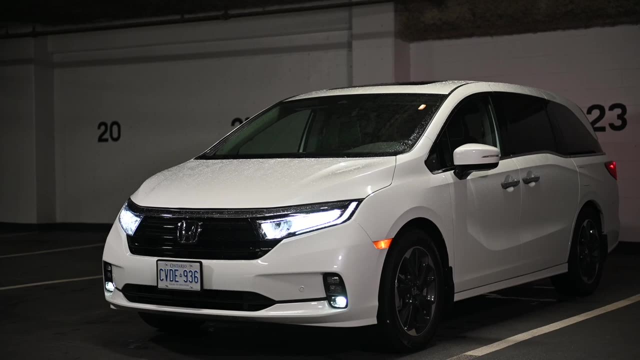 tolerances are like and whether or not the panels are aligned together. So we'll do a quick check on these things right now, And then I'll talk about the seven reasons why these things make more sense than SUVs. Okay, so first let's check the paint thickness using a paint thickness. 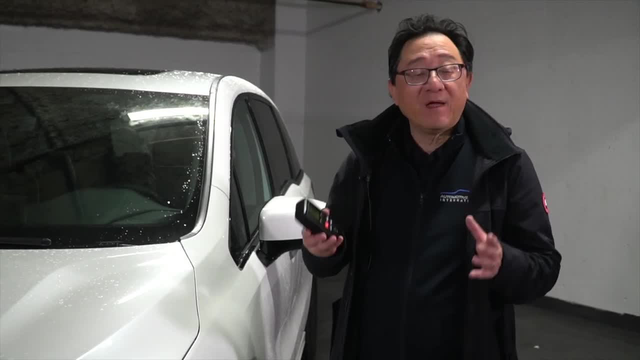 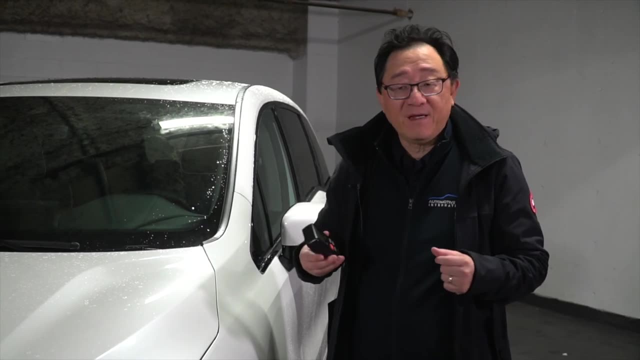 gauge And basically it should be between 100 to 180 microns. And the reason why this is important is because the thickness of the paint kind of indicates the overall quality of the paint. Thicker the paint, of course, the better. In the case of this, Honda Odyssey. 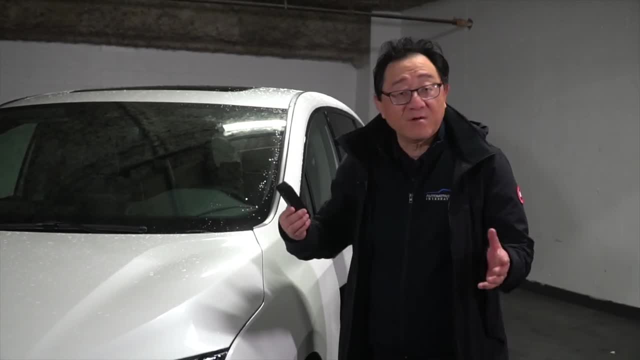 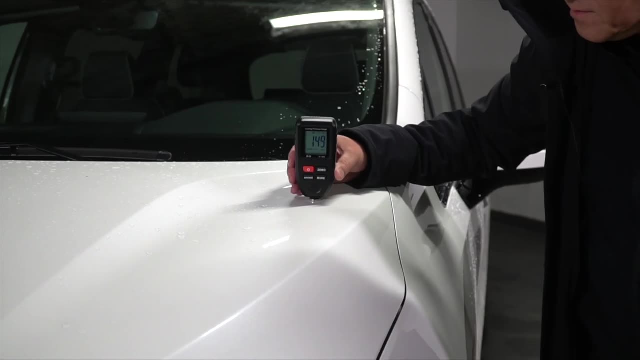 I'm actually surprised that it's a little bit thicker than normal, about 20% thicker than other cars. I've tested at about 150 micron in the front here 130 on the side, So it's also a little bit thicker. I did check all the way around And, generally speaking, on this Honda Odyssey. 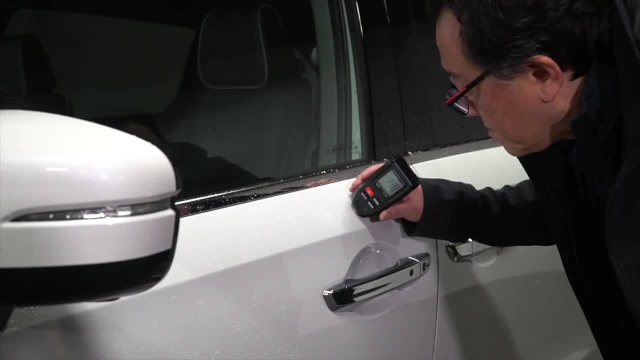 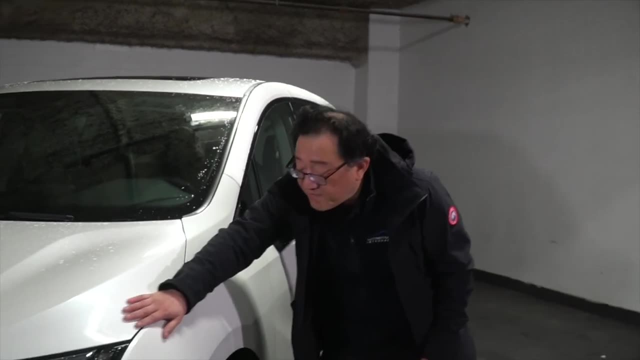 the paint thickness is between 130 and 150. So it's about 10 to 20% thicker than other cars I've tested, which is a good thing, And the paint quality when I checked it from front to back in terms of the gloss. 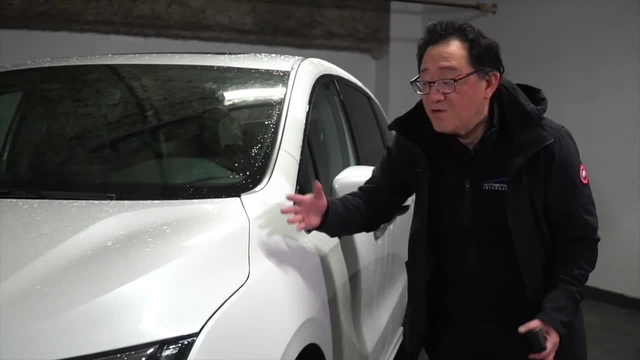 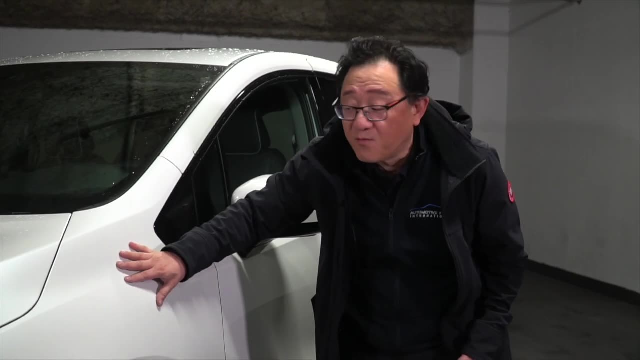 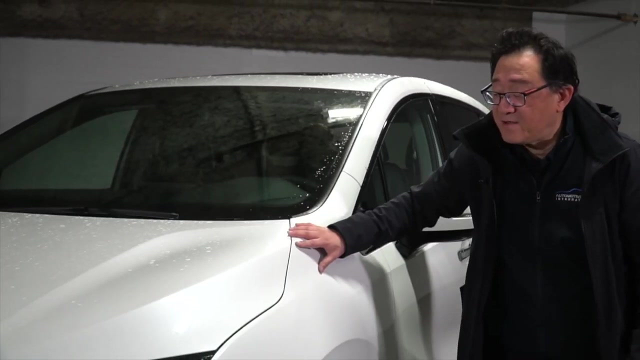 orange peel the amount of clear coat you know what. It's actually fantastic. I'm shocked at how good and how much of a first-class paint job they did with this Honda Odyssey. So super happy with the paint job. Now let's check to see if the body alignment and the panel fit. 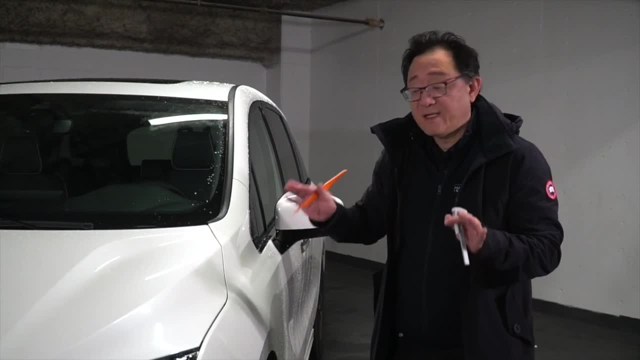 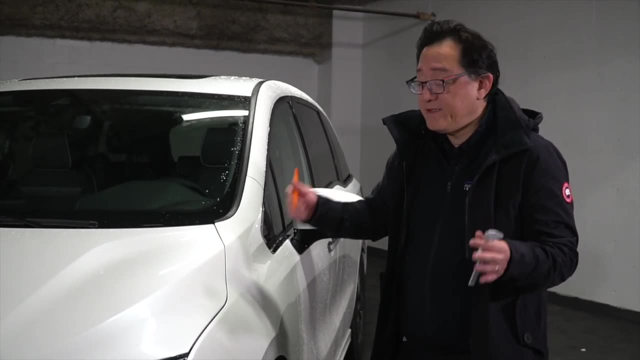 is as good as the paint job. So now we're going to check the body alignment and the quality of the fit and finish of all these different panels, And how I do that is simply to check for the consistency of the paint, And then I'm going to check the quality of the paint And I'm going to 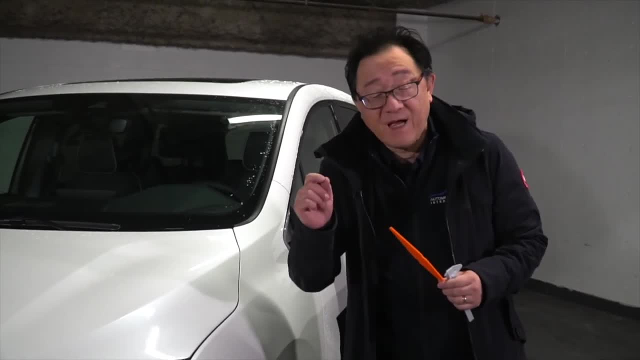 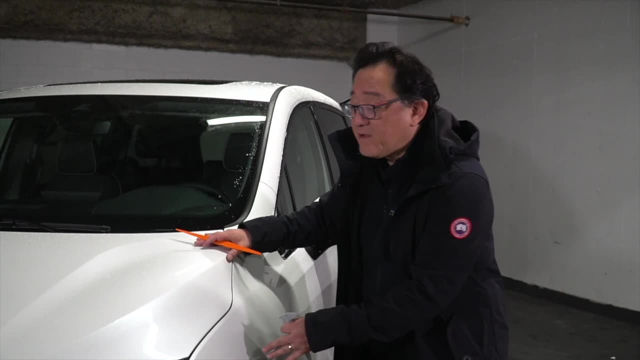 check the thickness of the gap and to see what the width of the gap is. So you want the gap to be sort of four to six millimeters, not much more than that. And the better fit the panels are, the more likely the better overall quality is for a whole car. So it's really important to test for. 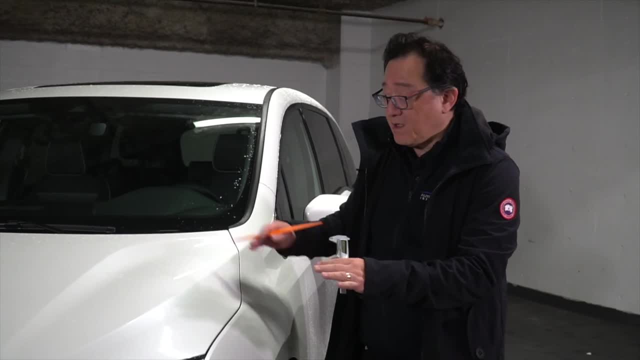 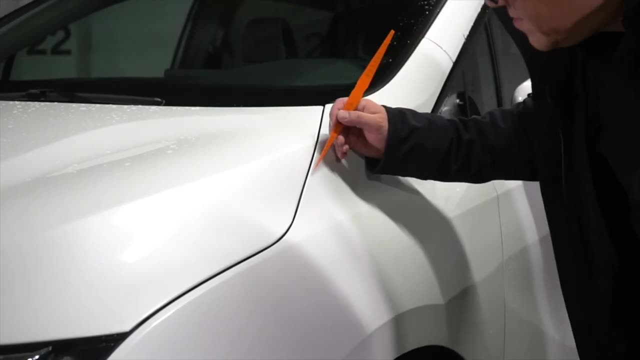 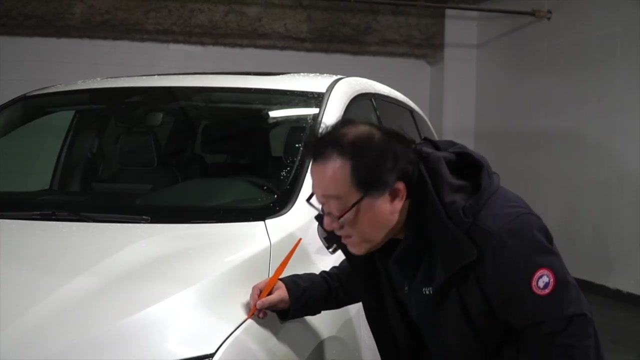 that I use a couple of different gauges here depending on which section of the car, But on this Odyssey I was actually quite surprised that in terms of the hood to the front fender ratio, it's best I've seen in the last two or three years. It's only about three and a half millimeter gap. 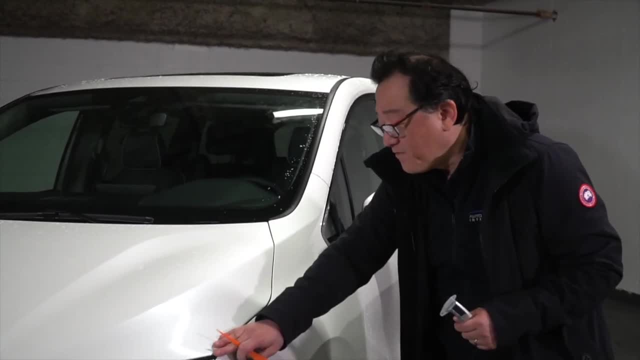 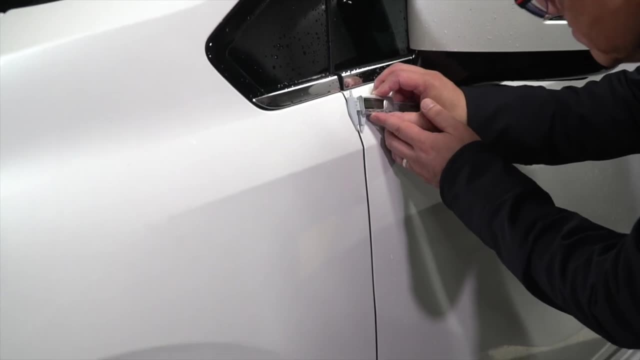 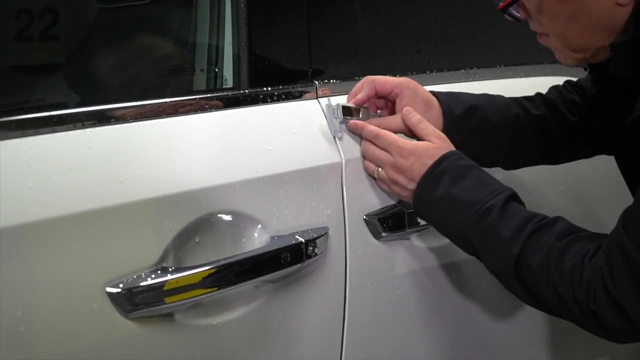 And it's almost a perfect fit from front to the back of the hood- Almost unheard of in this price range. And I also checked the width of the gaps in the door: It's about four millimeter here and about 3.9 millimeter here, and about the same for the rest of the door panel. So both in terms of 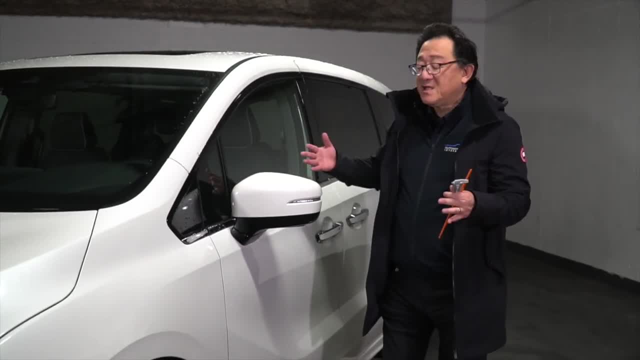 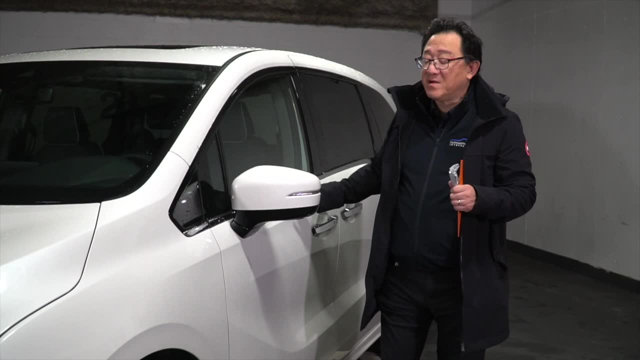 and body fit and finish and panel alignment. this is probably one of the best I've actually seen for many years, And so I'm very impressed with the manufacturing quality of this Honda Odyssey. Now let's get into the several reasons why I still think this Odyssey and the minivans in 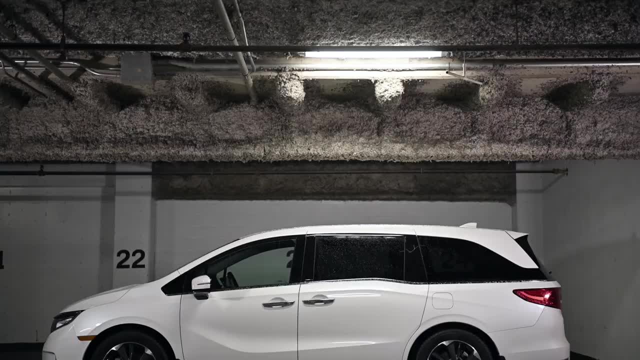 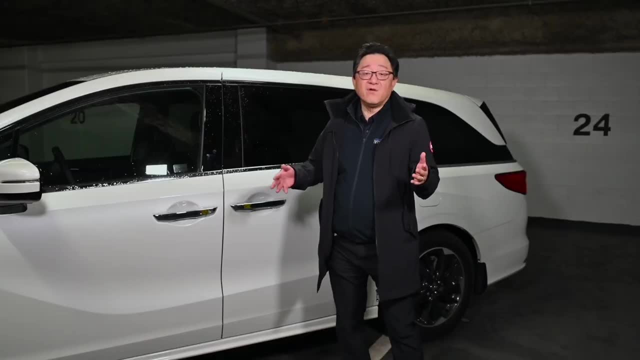 general, make more sense than buying your SUVs. As you know, most SUVs are based on car-based unitized body anyways. So when you look at SUVs, crossovers, station wagons and minivans, there aren't as much differences as you think anymore in terms of engineering anyways. But the 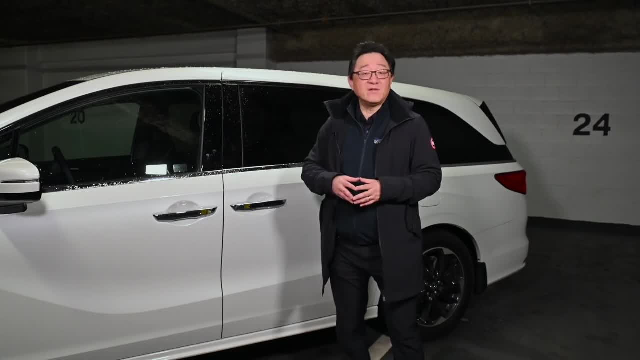 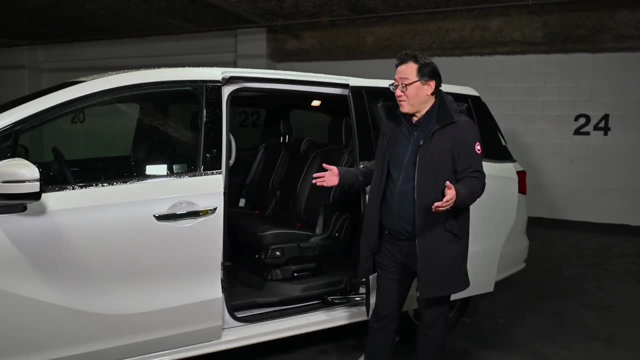 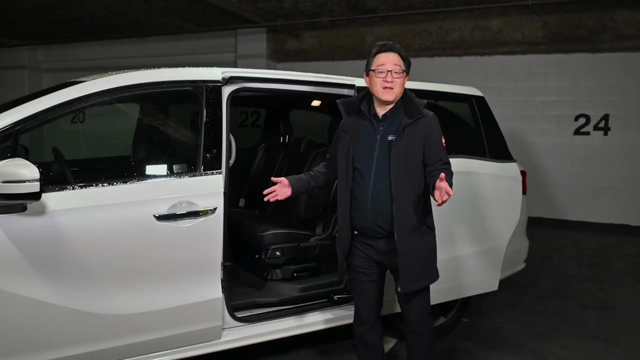 telltale sign that minivans are still a little bit different than SUVs is the sliding doors, which of course makes so much more sense from an engineer's perspective. I know this is what makes minivan look like minivan, And perhaps that is not necessarily a fun thing, because image is 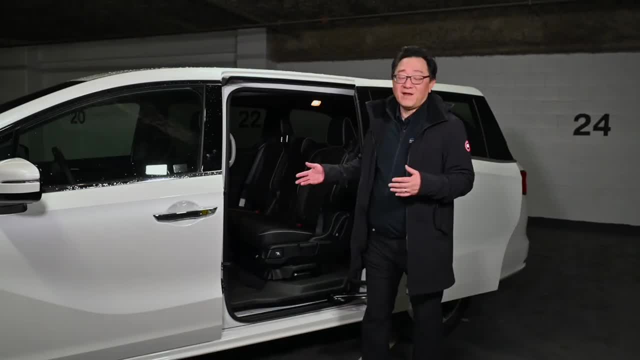 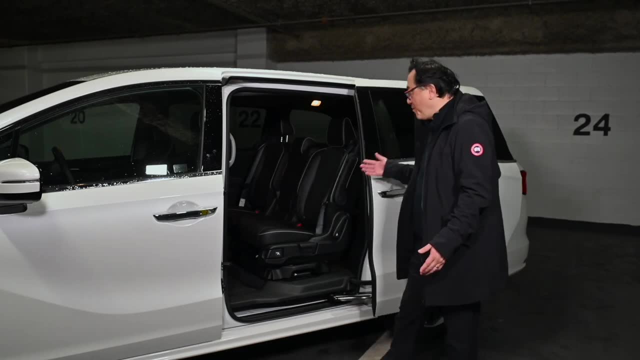 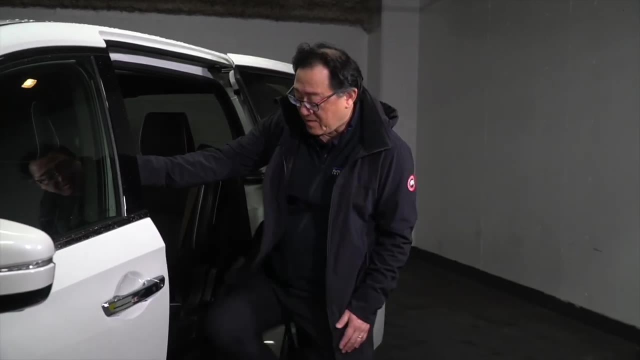 everything these days And a lot of people don't want to be associated with minivans, for whatever reason. I mean this makes so much more sense. It slides open. It doesn't swing open to another car beside it. It's wide opening so that it's easy to get in and out, like this. 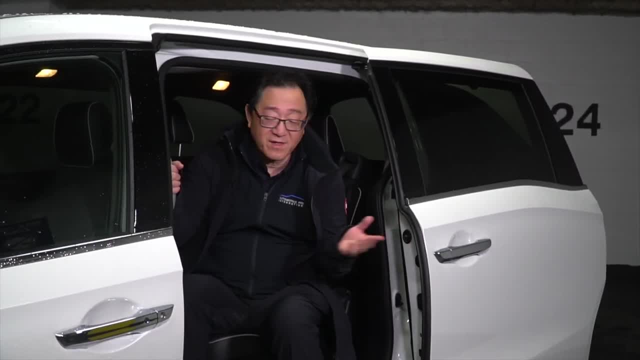 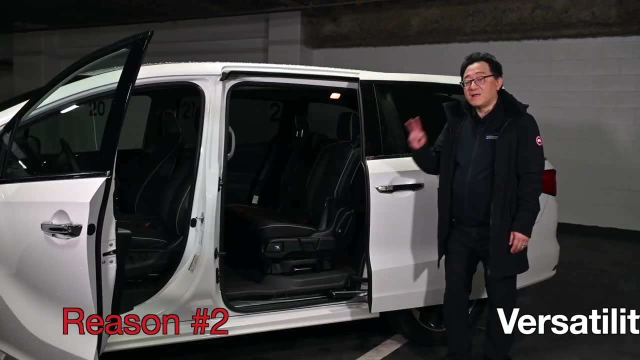 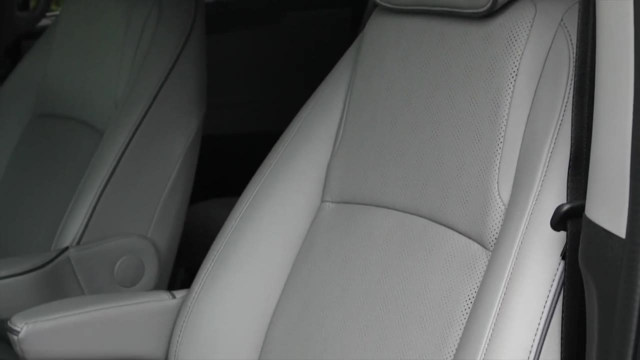 And for everyone, whether it's for adults or for kids. this is the reason why minivans make more sense than SUVs, or at least the first point. The second point is the practicality and the versatility of this minivan. Look how much space we get. The front seats are comfortable. 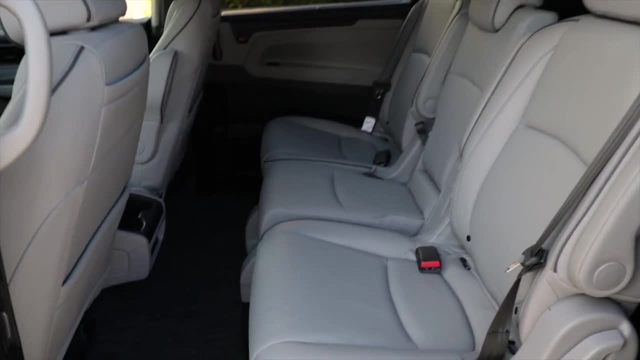 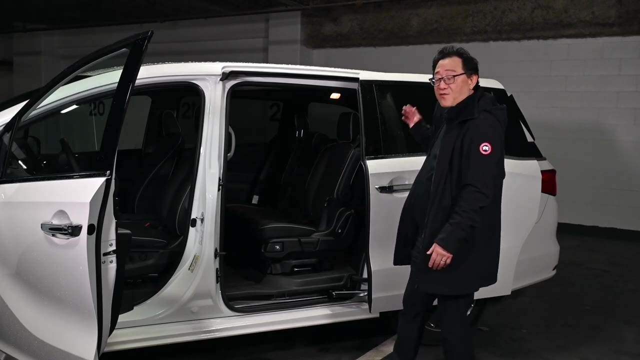 The second seats are super roomy and comfortable, with a flat floor, And even a third seat is super usable And even if you're a very tall person, you can actually sit in the third row and be comfortable. You cannot get that in most three-row SUVs. So this design and the way that it was, 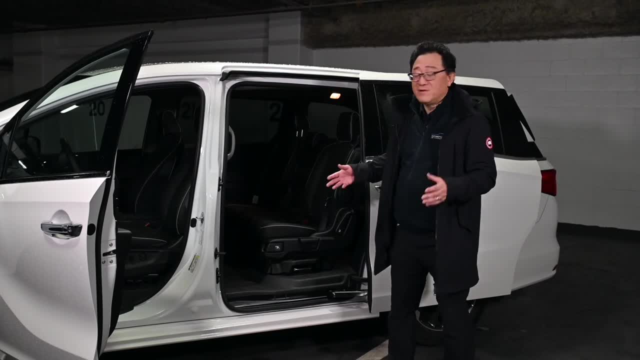 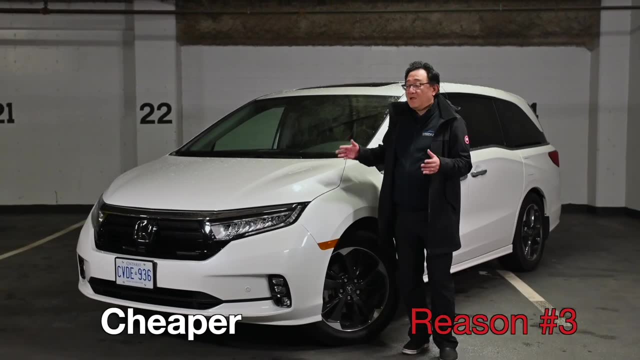 engineered to accommodate family and as a people mover, it kind of just makes sense. The third reason why minivans like this Honda Odyssey makes more sense is simply because you get more value for money. And the third reason why minivans like this Honda Odyssey makes more sense. 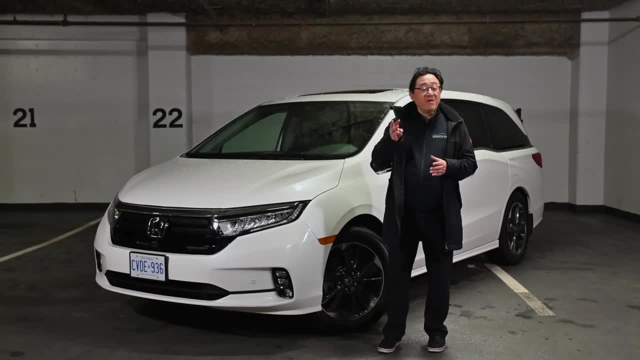 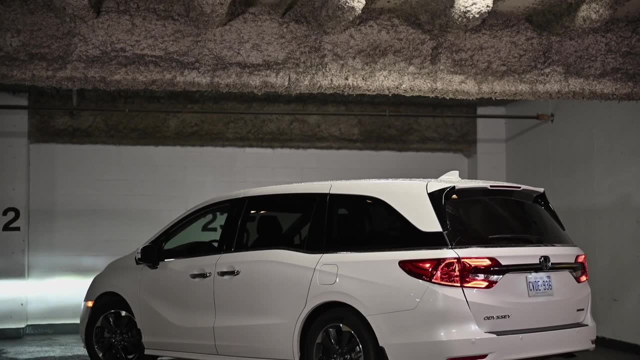 is simply because you get more value for money. It's cheaper than most SUVs that have three rows because they moved upscale and you get lots of features and lots of content. So it really is a value leader in terms of buying a family or people mover. The fourth reason why I really like this: 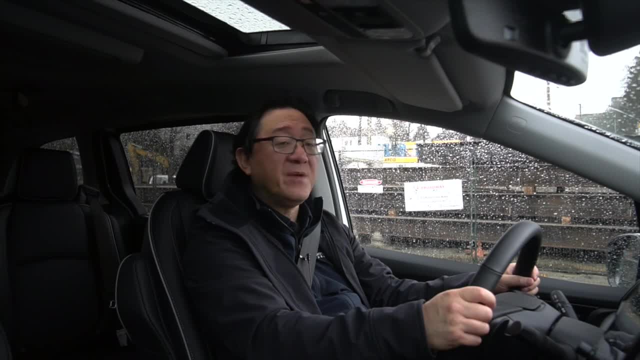 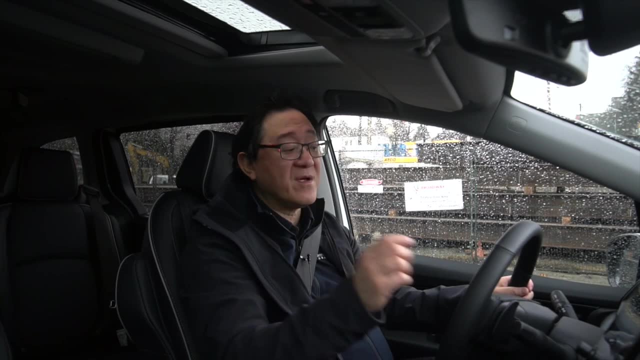 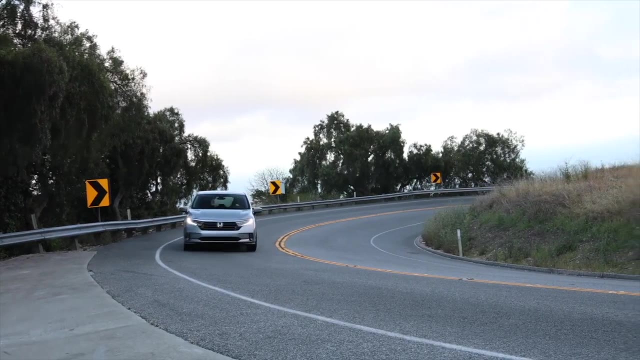 Honda Odyssey as a minivan is simply because it drives better than most SUVs. It's very agile, has a good road feel, the steering is just right and almost kind of feels like a sports sedan, Compared to larger SUVs that are sometimes bumpy and difficult to drive and not 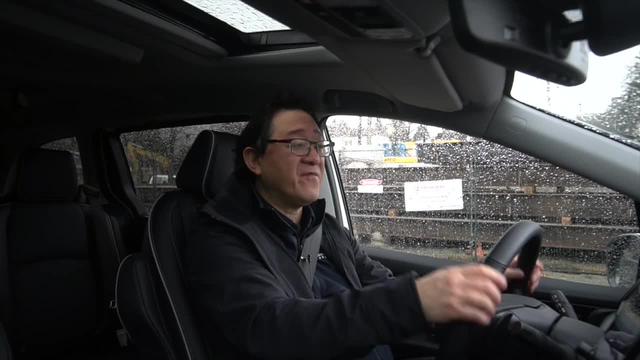 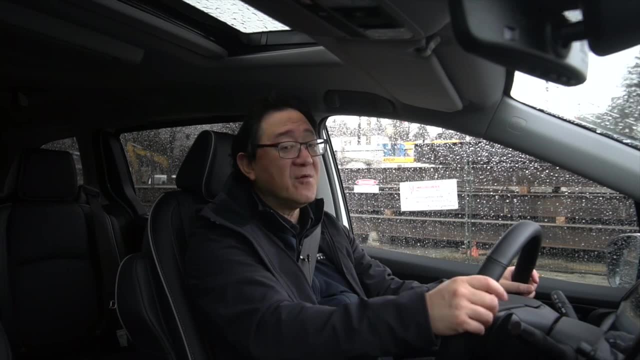 all that fun to drive. in fact, this thing is way better. In fact, if you were to ask me, would I prefer to drive a big SUV or this one as a daily driver? I'm going to take this one for sure, because it's actually quite fun to drive and I'm really enjoying it. Good braking. 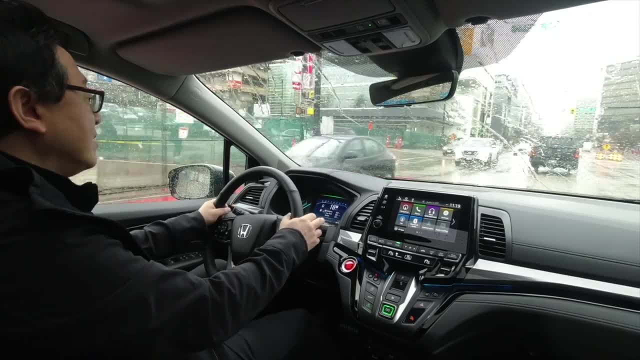 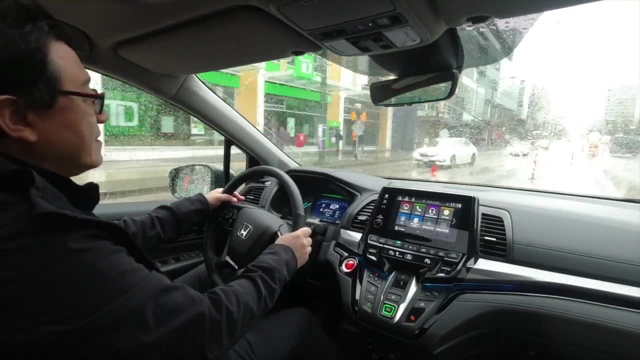 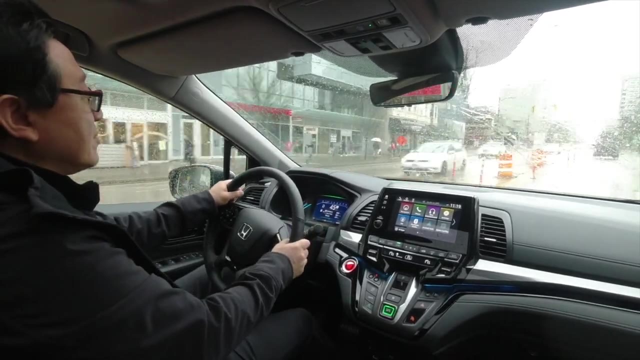 really good: engine feel, solid, transmission shifting, You know what- Really well engineered from the Honda side and I think this thing will outrun most SUVs and even larger three-row crossovers out there. So fun to drive factor is definitely one reason why. 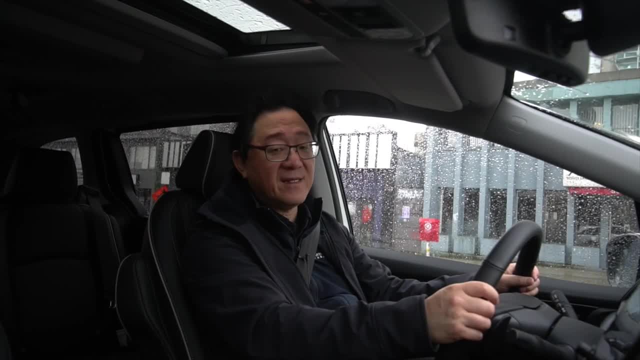 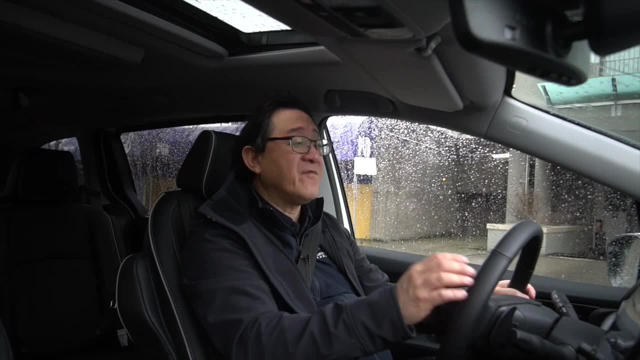 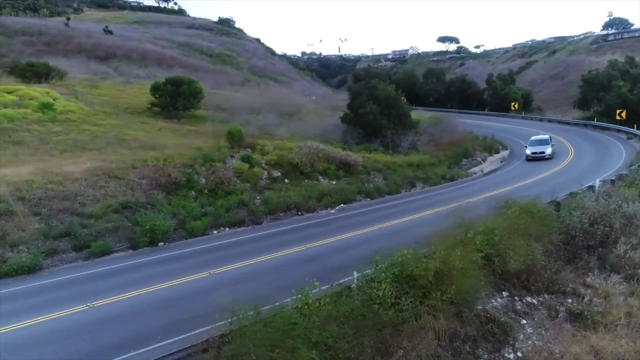 the Honda Odyssey and minivans simply makes more sense. The fifth reason why this Honda Odyssey makes sense is kind of related to the fourth reason, which is the fact that it rides really well. It's ultra smooth, very comfortable, Quiet, almost like a luxury car. You know what? It's kind of almost like a Lexus level. 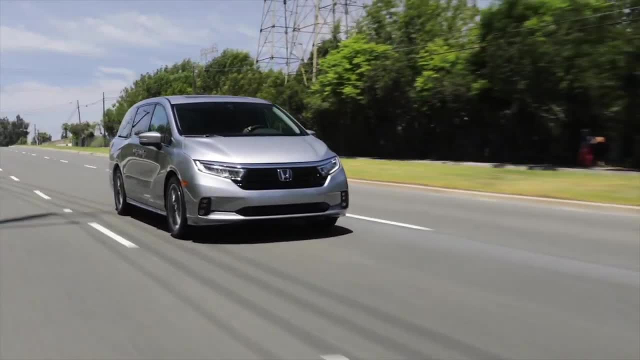 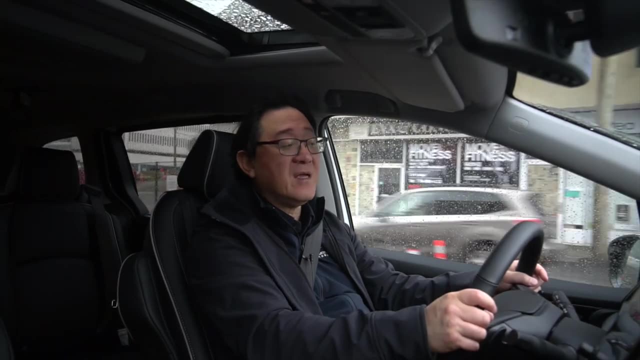 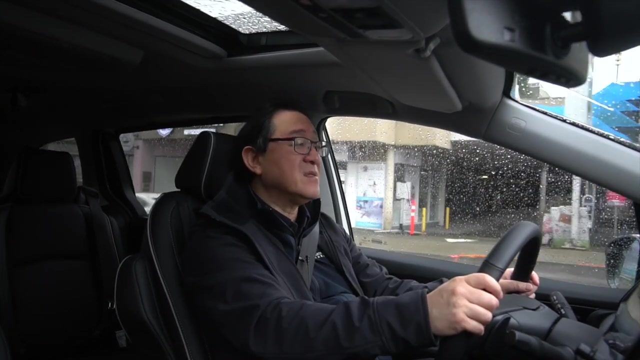 of ride and drive feel So. for passengers especially, they're going to love being in this Honda Odyssey. compared to a large SUV that's sometimes very bumpy and not all that comfortable, especially over rough roads, This thing is definitely better overall, So I think it's. 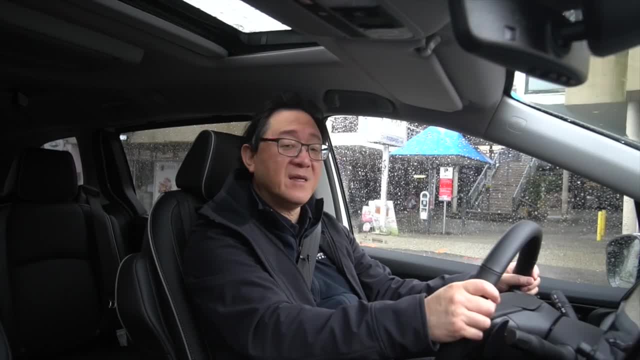 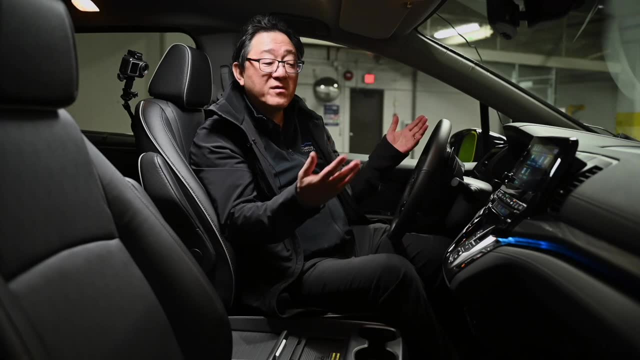 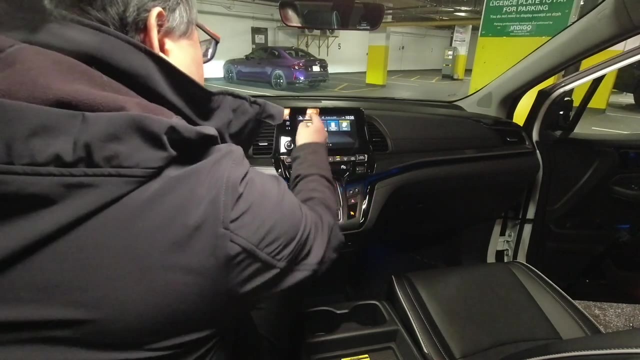 more comfortable. It drives better. It just kind of makes sense. The sixth reason why minivans makes sense, especially this one here, the Honda Odyssey, is because you get cool features that are typically not available on other SUVs. So, for example, we get two features here called cabin watch and cabin talk. Cabin watch is very 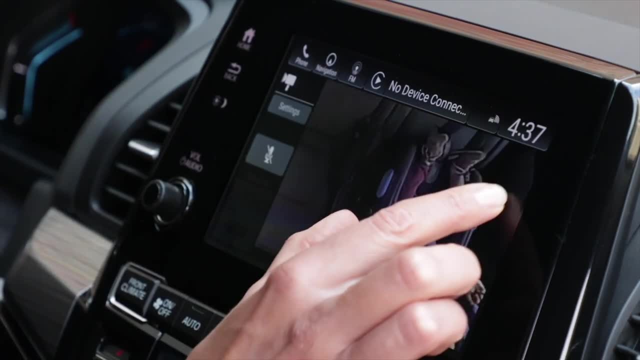 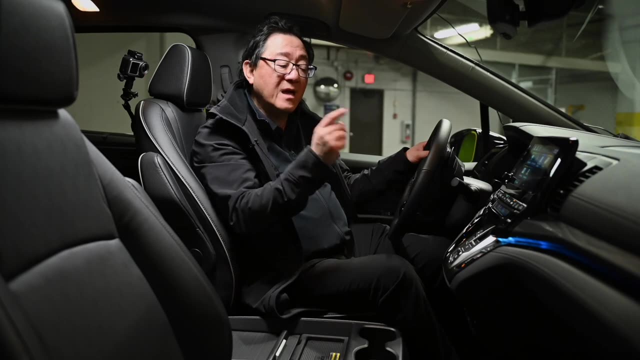 simple. It's basically kind of a bird's view perspective of the second row and the third row So you can see what's going on in the back for your kids or whoever else is sitting back there. And then cabin talk is when your voice is amplified so that 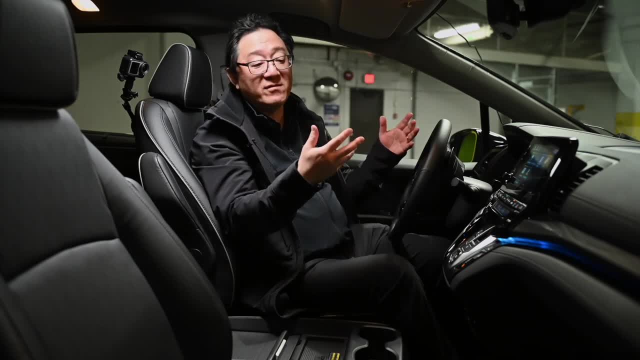 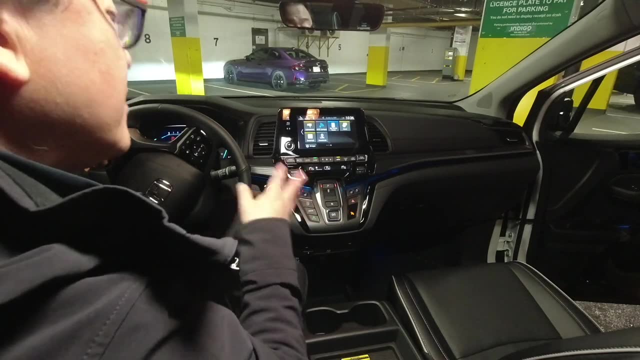 people can hear from the back without you speaking loudly, So that allows you to have a conversation and people can actually hear you clearly. And these features are typically not offered in other SUVs, but you do get them. in the Honda Odyssey You can even flip the third. 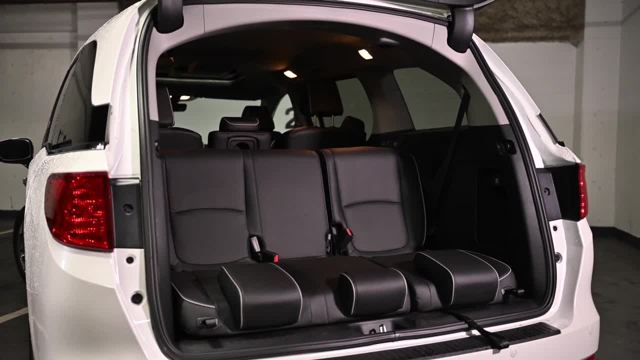 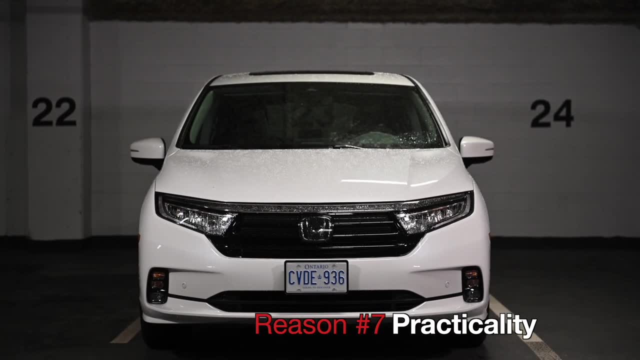 row seat at the back, So it kind of becomes like a tailgate party. So those are some of the cool features I find in this Honda Odyssey. The seventh reason why I like minivans like this Honda Odyssey better than SUVs is simply because there are lots of practical designs.